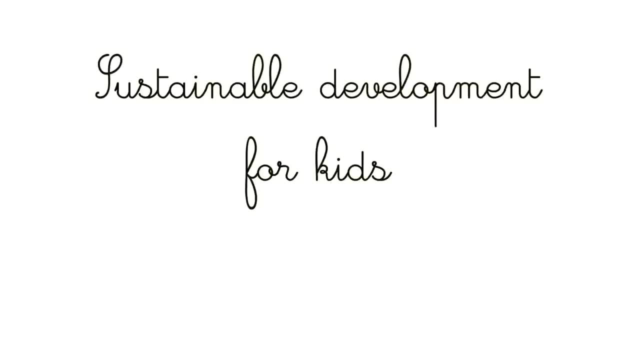 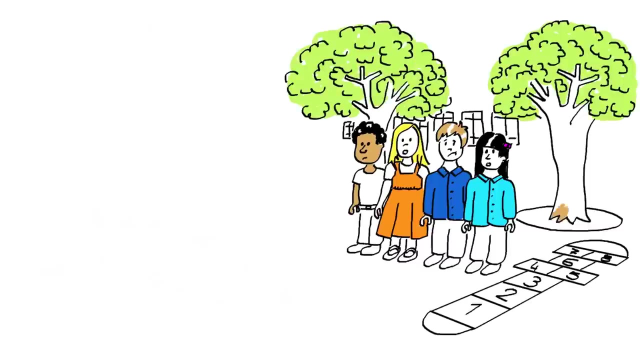 Hey kids, did you hear about the grade 3 class who partnered with Eco Man to beat the dreaded Dump It Man to make a better world? Check it out. It all started out as a normal day, but when the children arrived at school, the playground was filled with garbage and on. 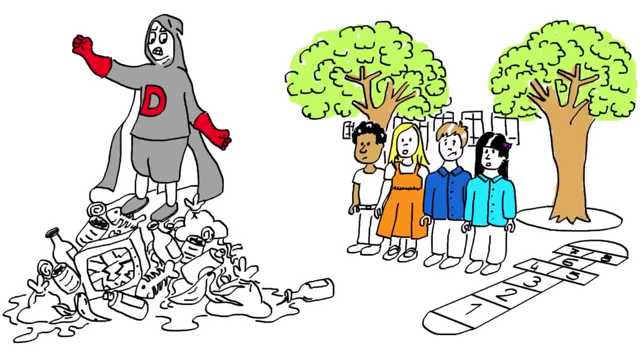 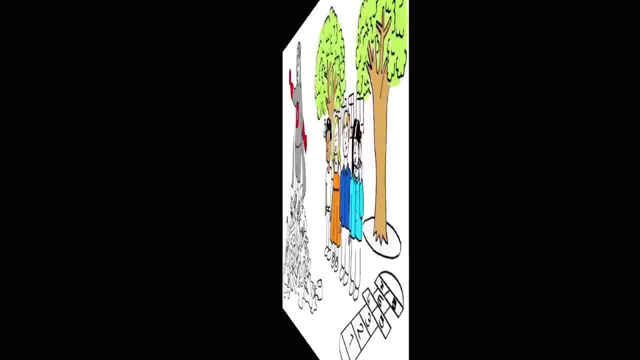 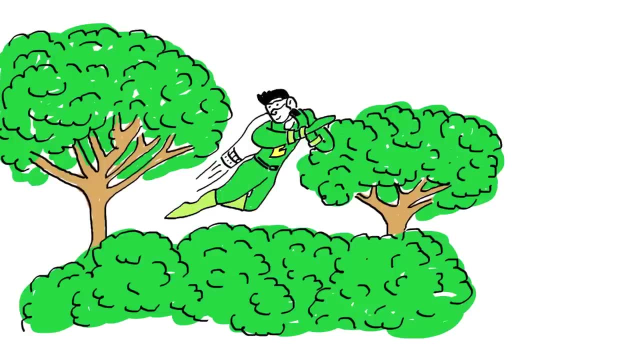 top of it stood the dreaded Dump It Man Gross. What to do. The class had been studying how to be green, so they knew to call their friend Eco Man. Eco Man was busy protecting the Amazonian rainforest, but he was able to arrive in just a few seconds, thanks to. 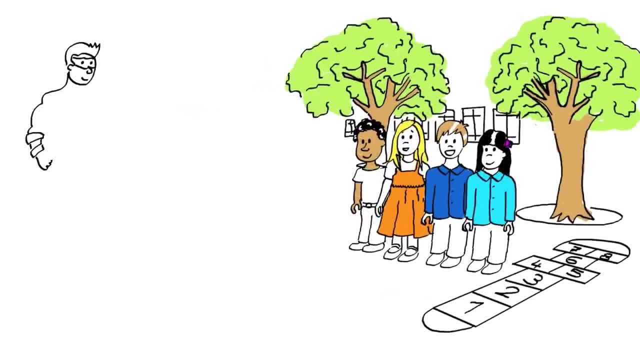 his renewable energy jet pack. Hey, Eco Man, cried the class. What's going on here? Eco Man looked around. Ah, he said someone has been duped into Dump It. Man, If we don't want the whole world to look like this, we have to recycle. Luckily, we. 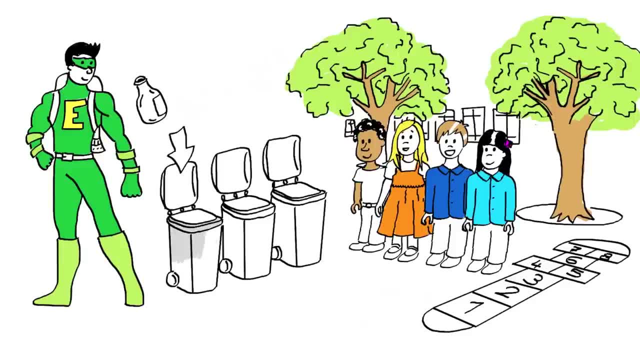 have a system to do this. Different waste goes into different bins: One for glass, one for plastic, one for cardboard and newspapers and one for everything else. If we do this, then glass can be melted and made into new glass, paper can be recycled and plastic 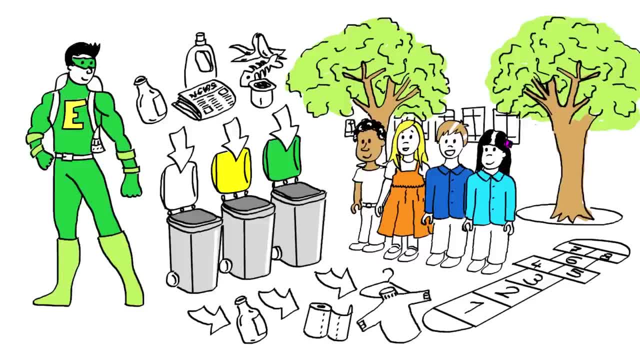 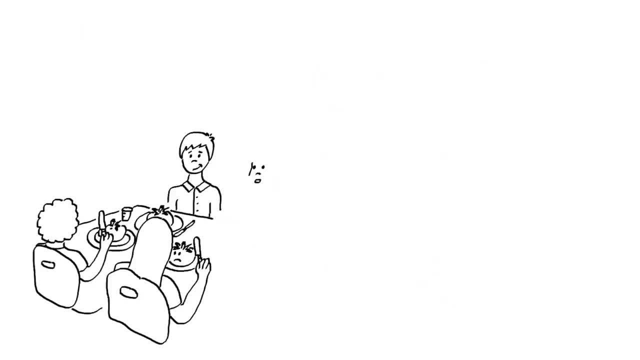 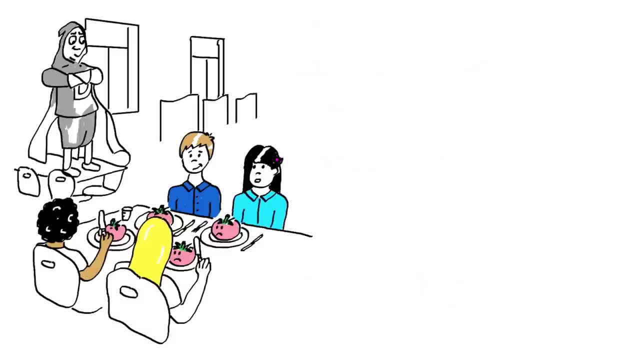 turned into hangers, bottles or even a new sweater. Thanks Eco Man. the class shouted. Later that day the class sat down to have lunch and found pale, tasteless tomatoes on their plates. They could see the dreaded Dump It Man sneering in the corner, so they called. 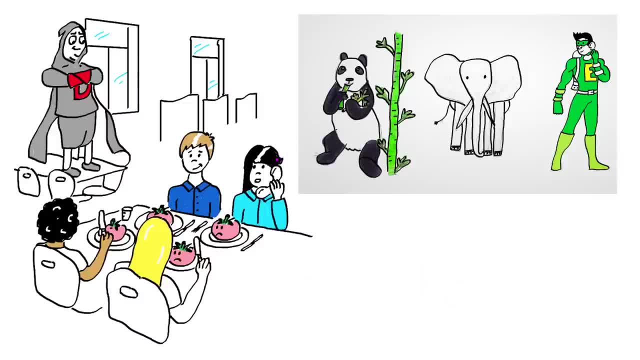 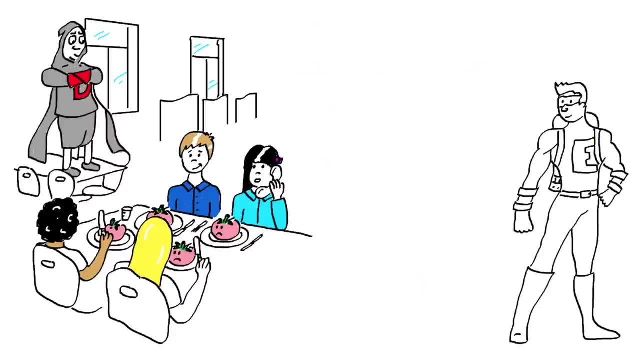 Eco Man again, who was busy protecting endangered animals. Hey, Eco Man, what's going on? Eco Man explained that the Earth gives us fruits and vegetables all year round, but different ones grow in different seasons. For example, rhubarb comes in the spring. 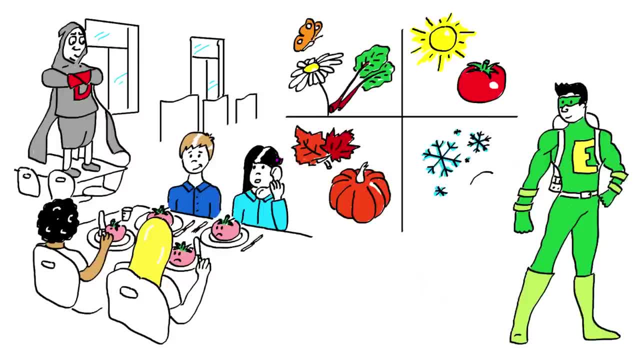 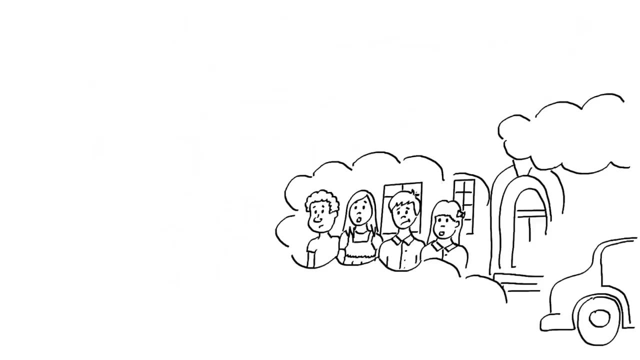 tomatoes in the summer, Pumpkins in the fall, and in the winter we get carrots. And when we respect natural cycles, nature helps us, For example by giving us ladybugs who eat the aphids who would otherwise eat our plants. Yay, nature. At the end of this strange day, the children left school.